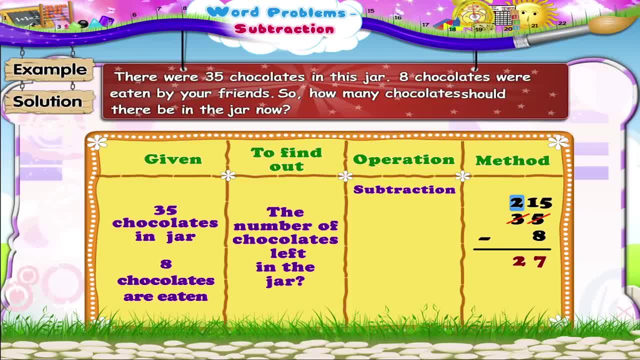 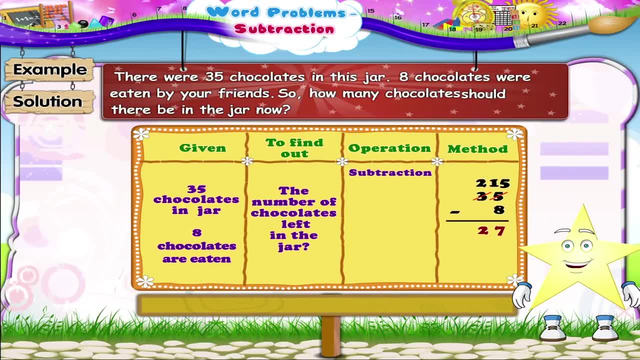 Two tens remain. as it is, The answer is 27.. So, Starry, now tell me How only 27 chocolates are left in this jar. See, Starry, just like addition, we can also make use of subtraction in our everyday life. 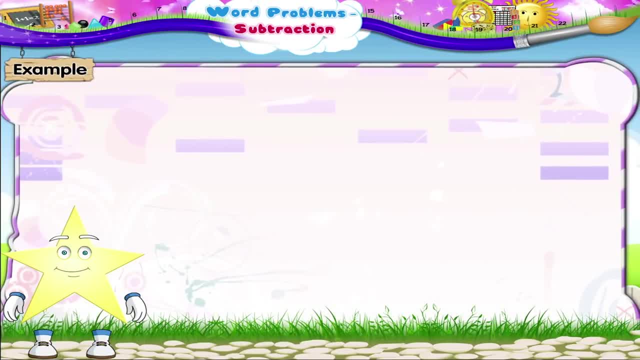 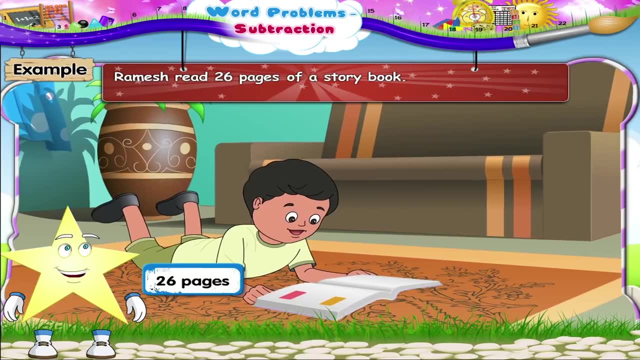 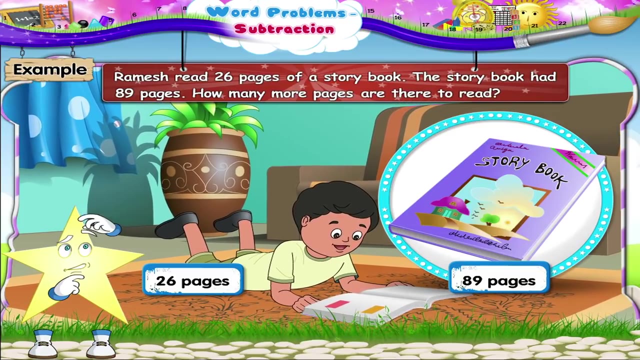 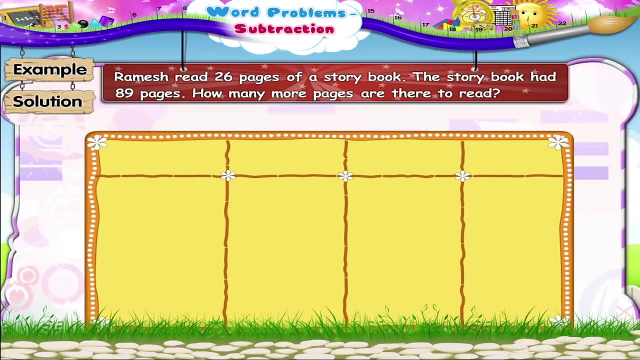 Let us take a look at the next example. Ramesh read 26 pages of a storybook. The storybook had 89 pages. How many more pages are there to read? Remember, Starry, just like addition problems, first find out what is given. 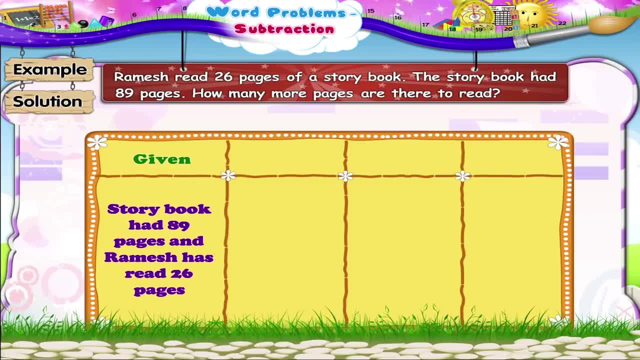 Here it is. given that the storybook had 89 pages And Ramesh has read 26 pages, What do we have to find? Yes, we have to find the number of pages left to be read, So we shall subtract 26 from 89.. 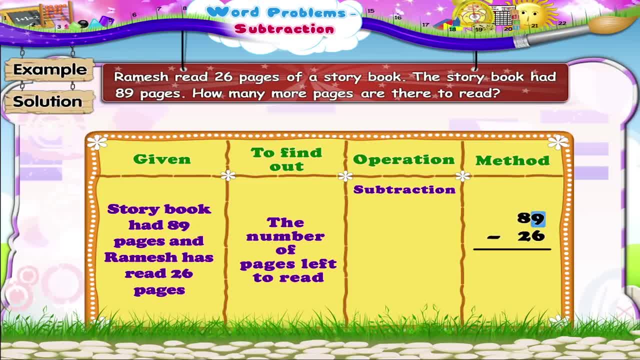 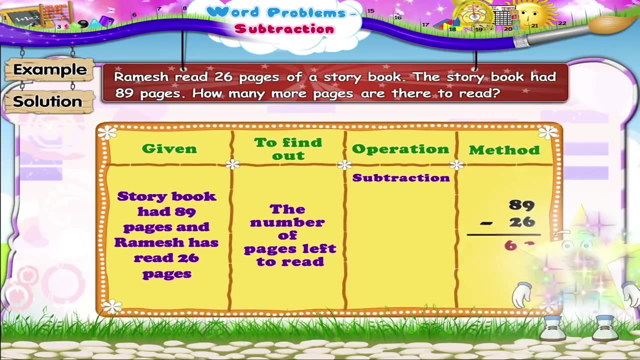 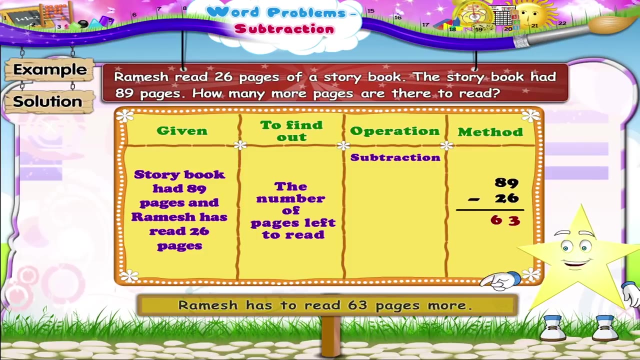 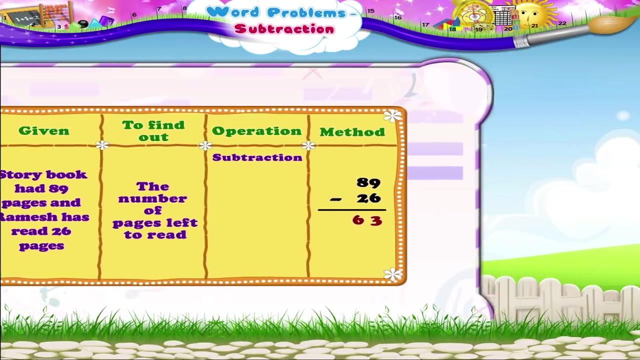 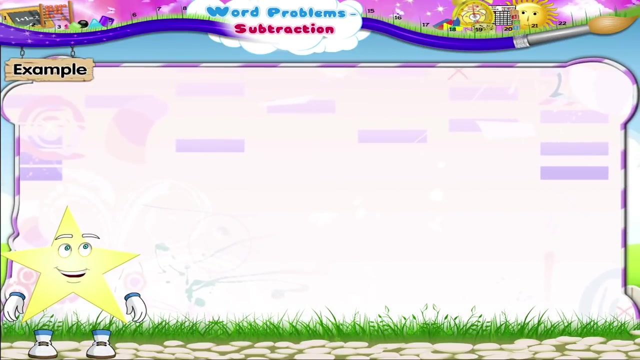 9 units minus 6 units is equal to 3 units. 8 tenths minus 2 tenths is equal to 6 tenths. So Starry Ramesh has to read 63 pages more. Let us solve the next word problem, Starry. 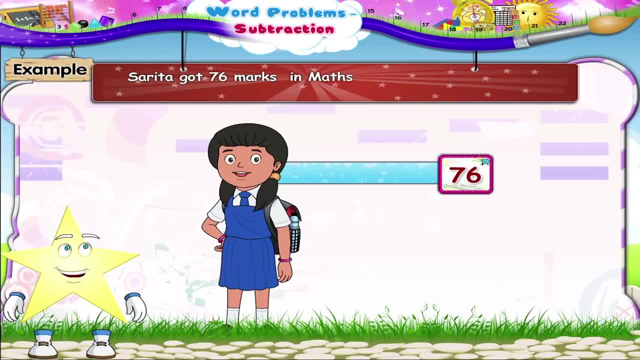 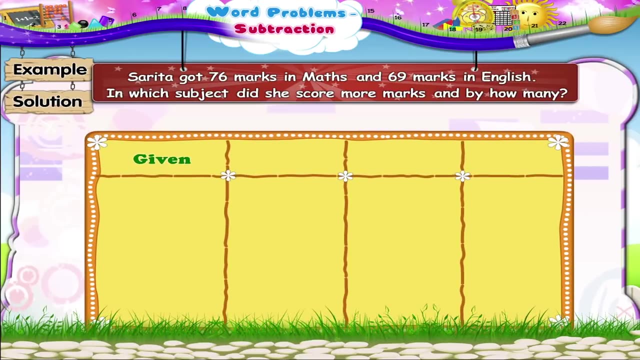 Sarita got 76 marks in maths and 69 marks in English. In which subject did she score more marks and how many? What is given here, Starry? Yes, it is given that Sarita scored 76 marks in maths and 69 marks in English. 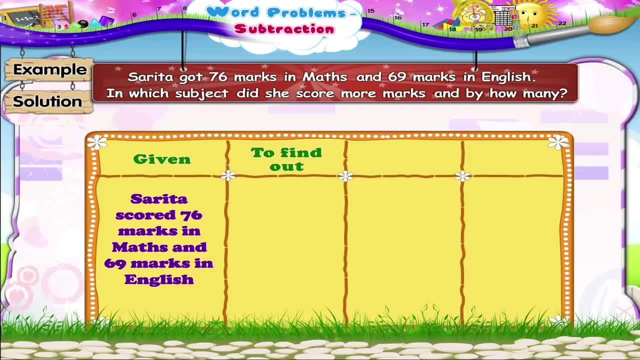 What do we have to find? Yes, we have to find the subject in which Sarita scored more marks. That's easy. Sarita has scored more marks in maths. Let us find out how many marks more. For this, we shall subtract 69 from 76.. 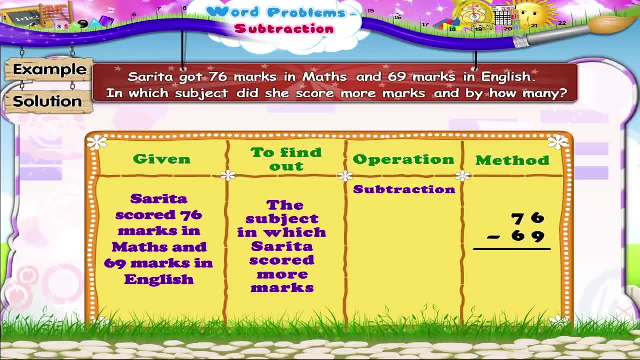 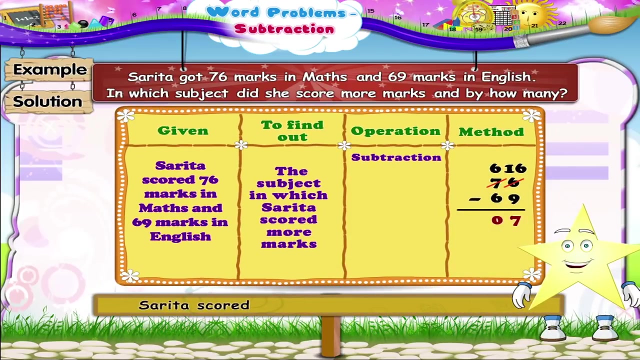 so starry. what should we do first? yes, subtract 9 units from 6 units. is that possible? no, so we borrow 110, that is 10 units. now, on subtracting 9 units from 16 units, we get 7 units. next, 6 tens minus 6 tens is equal to 0. thus Sarita scored 7 marks more in. 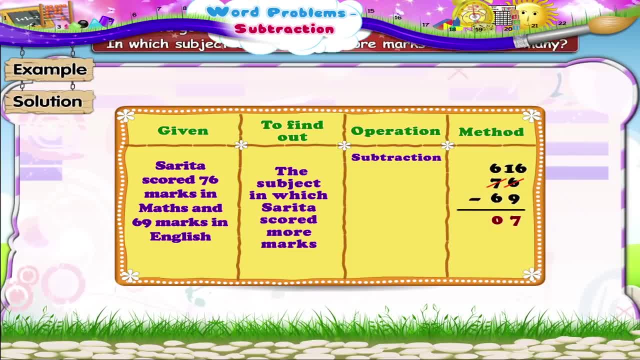 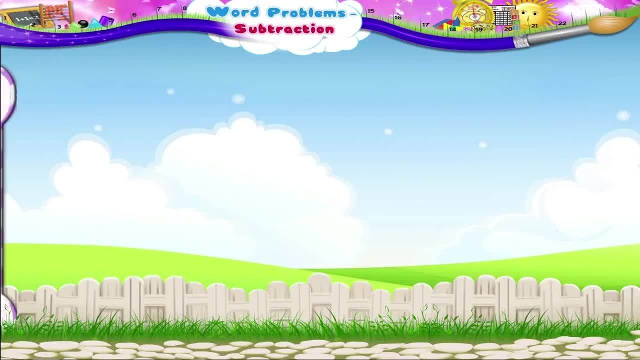 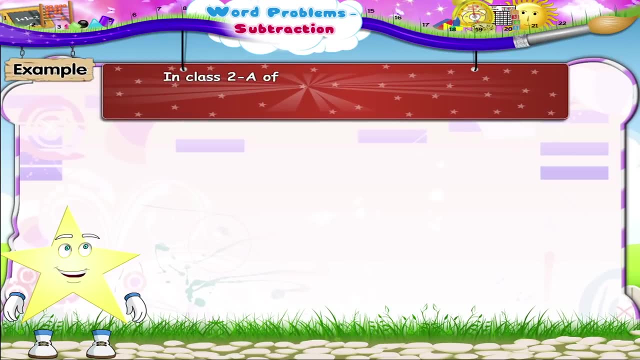 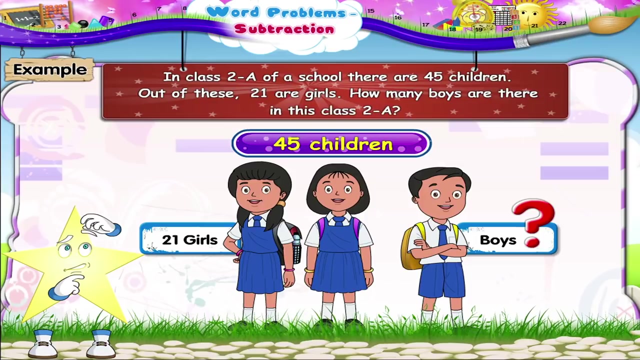 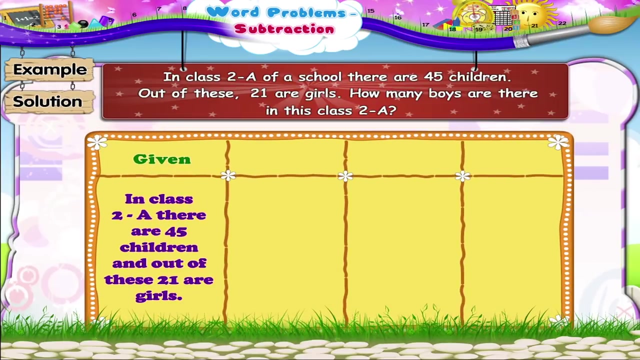 maths than English. come on, starry. let us solve the next example. in class 2- 2A of a school there are 45 children. Out of these 21 are girls. How many boys are there in this class 2A Here? it is given that in second A there are 45 children And out. 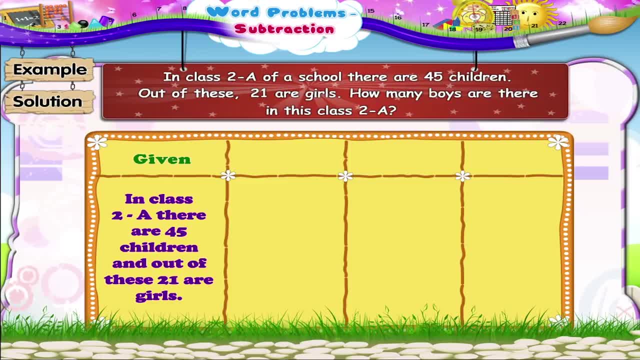 of these, 21 are girls. What have we to find out, Starry? Yes, we have to find the number of boys in second A. Will you solve this one, Starry? Yes, we have to subtract 21 from 45.. 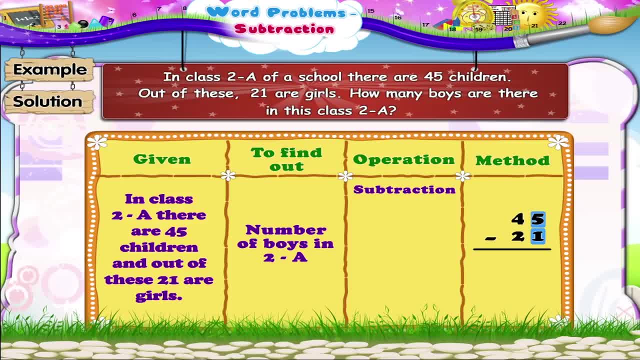 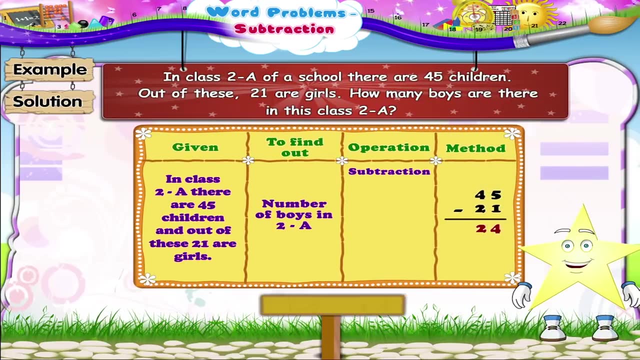 So 5 units minus 1 unit is equal to 4 units. 4 tenths minus 2 tenths is equal to 2 tenths. You are right, Starry, There are 24 boys in class 2A.